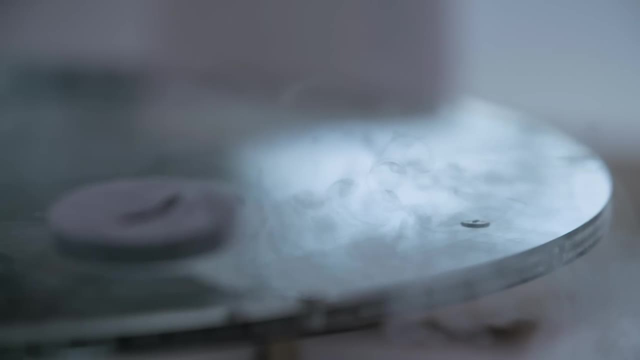 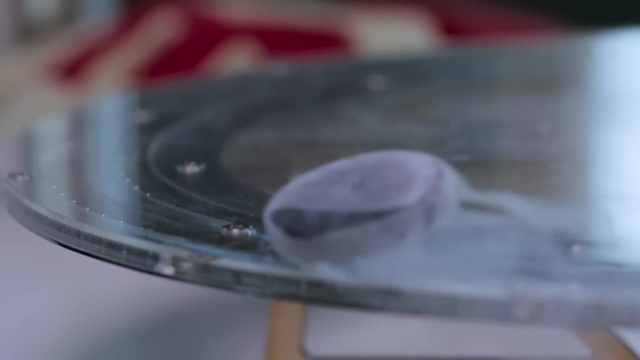 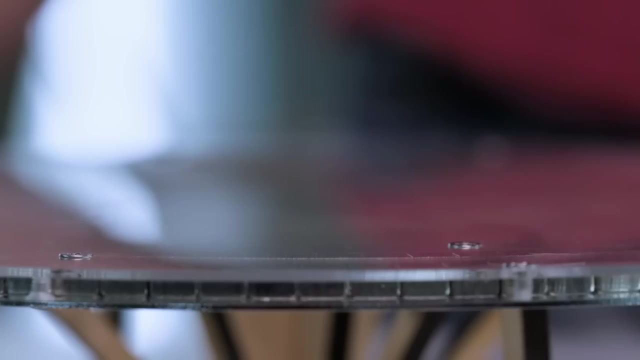 The latest claim of a room temperature superconductor set researchers around the world racing to replicate the findings, but yet again the claims appear to be false. So how do superconductors work and why are we struggling to unlock the next stepping stone in human technological progress? Let's delve deeper into what superconductivity is. 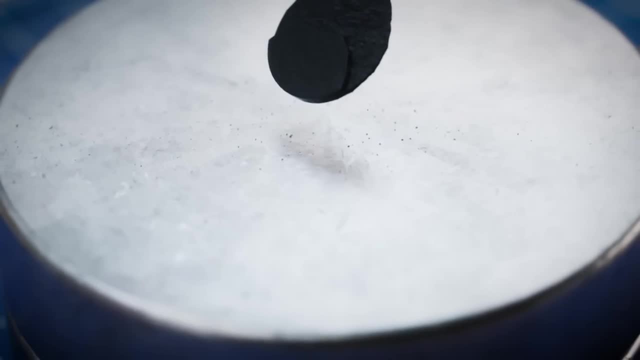 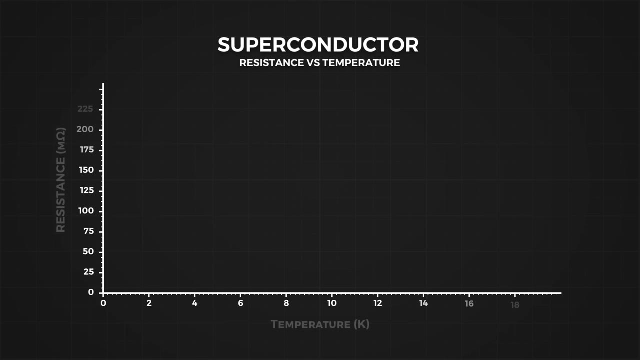 What superconductors are their current applications and what exciting prospects the future may hold for these remarkable materials. Temperature affects all metallic conductors with resistance gradually lowering with temperature, But superconducting materials are special in that their resistance drops to zero. 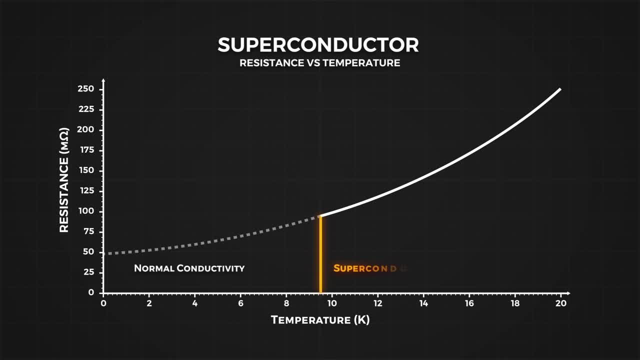 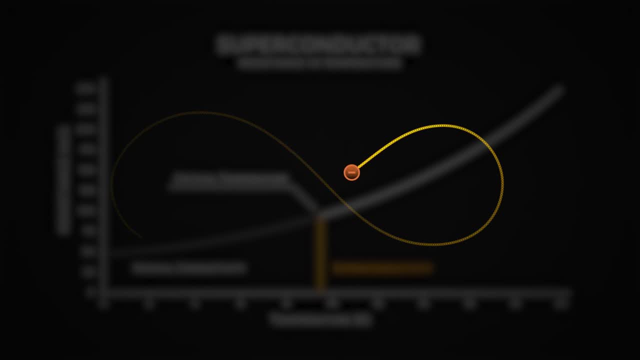 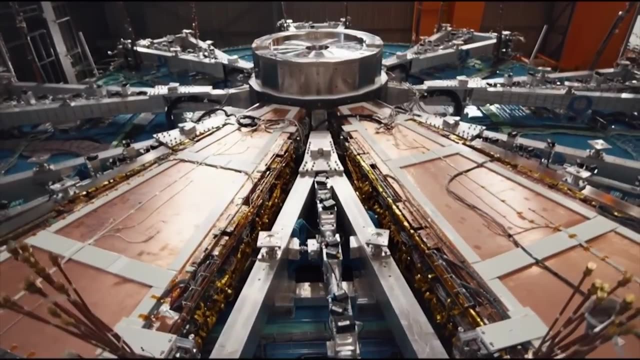 at temperatures close to minus 273 degrees Celsius, the critical temperature. In theory, when this happens, an electric current could travel in a loop of superconducting material indefinitely, never needing a power source. While we can't truly measure indefinitely, there have been practical instances where superconducting currents have flowed uninterrupted. 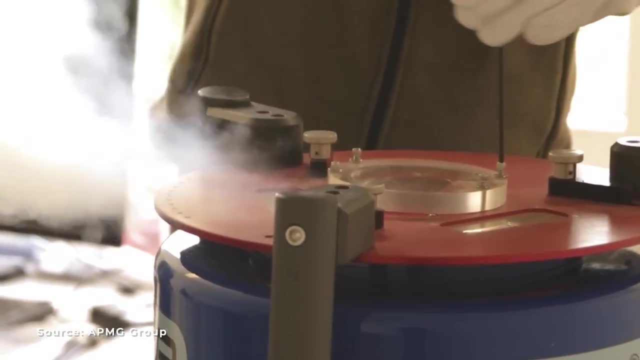 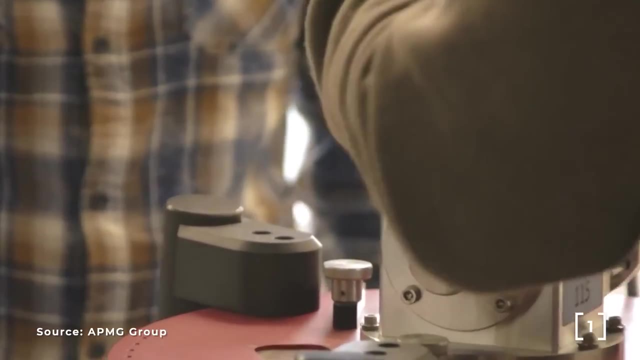 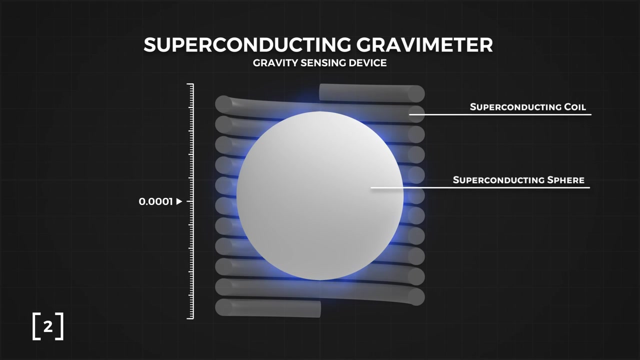 for decades. Here in Belgium, a superconducting sensor is being used to measure gravitational forces and has been in operation for over 28 years without any loss of current. It works by levitating a superconducting sphere in a superconducting coil in a stable position. Then we can track its position, and to do so, we have to measure the current of a superconducting sphere. We can measure the current of a superconducting sphere and we can measure its current and we can measure its position and we can measure its current and we can measure its. 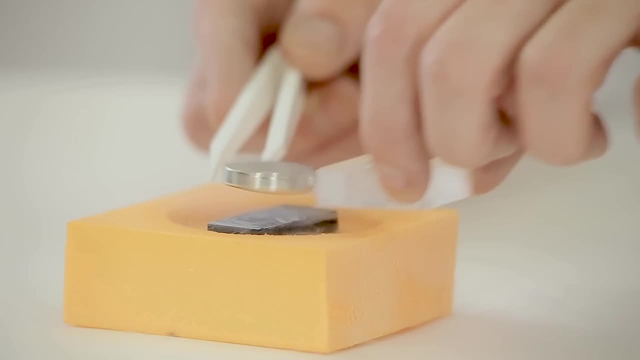 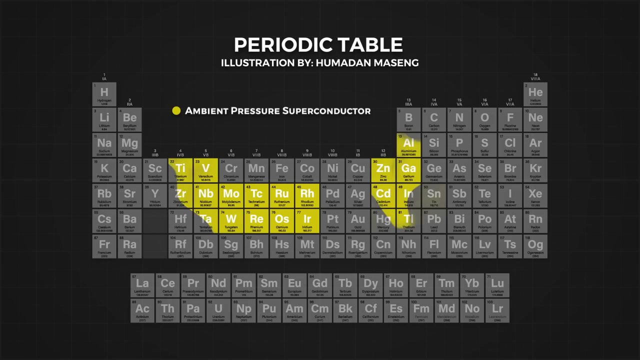 which changes with gravitational forces. Superconductivity is more common than you'd think. A little under half of the elements on the periodic table exhibit superconductivity. at low temperatures and when combining elements together or increasing their pressure, even more materials exhibit the phenomenon Initially. the underlying mechanism behind 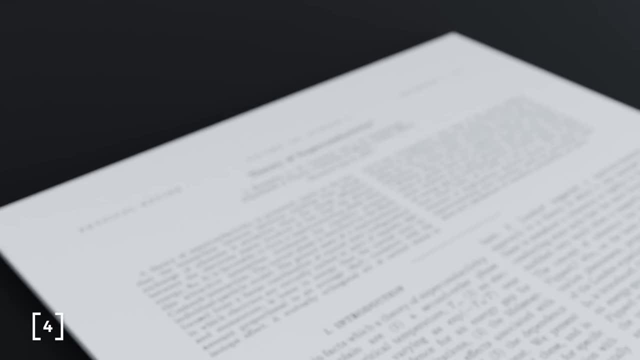 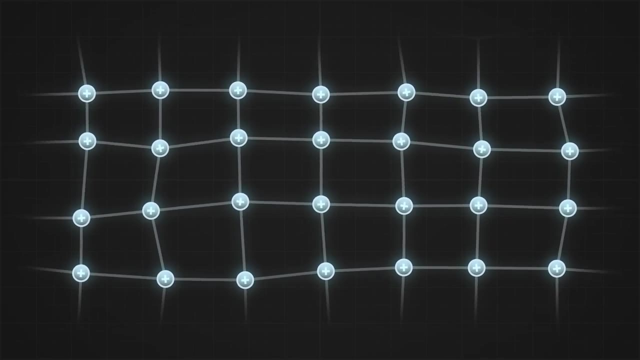 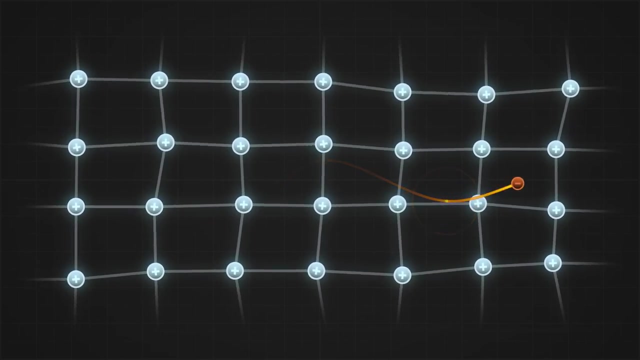 superconductivity was a mystery. however, in 1957 three scientists explained it in this ground breaking paper. At any temperature above absolute zero, all molecules shake a little. This means that electrons in a conductor slow down as they bump into the shaking crystal molecules. 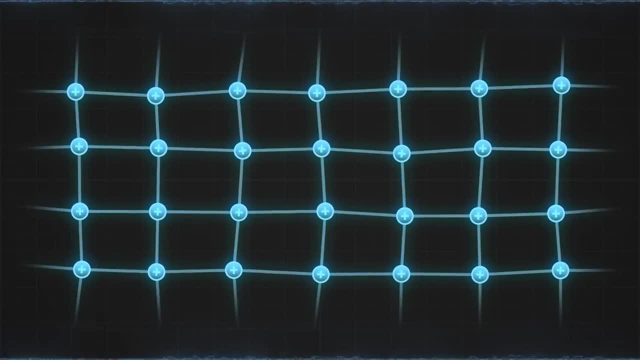 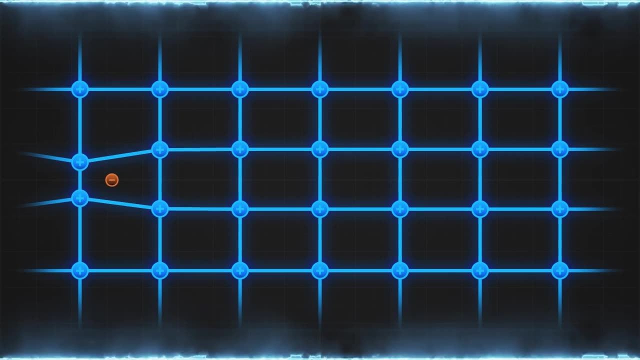 This is why conductors have some resistance, But at ultra low temperatures crystal lattices in superconductors vibrate less slow enough to allow one electron to draw nearby atoms together, creating a positively charged region that attracts another electron. This enables electrons which 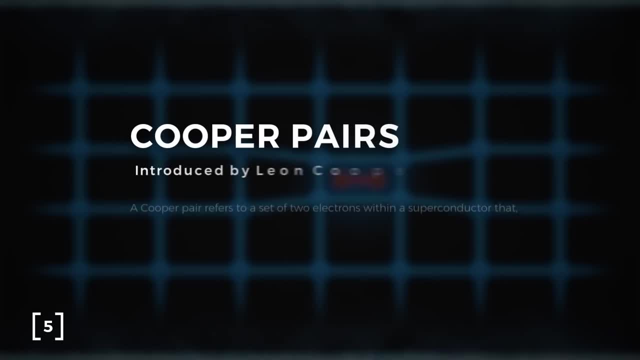 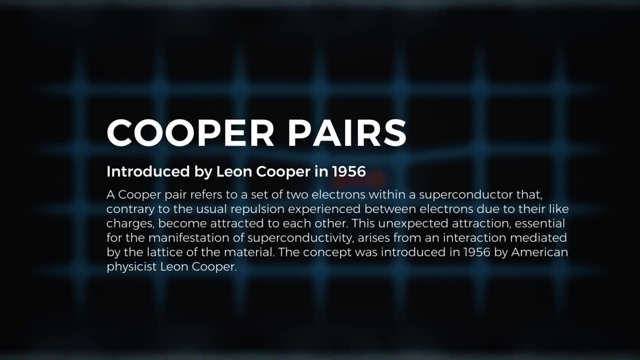 usually have a higher temperature than superconductors to vibrate. at a lower temperature, Electrons usually repel each other to interact and form pairs over nanometer scaled distances, known as cooper pairs. Electron pairs in superconductors behave as a single cohesive. 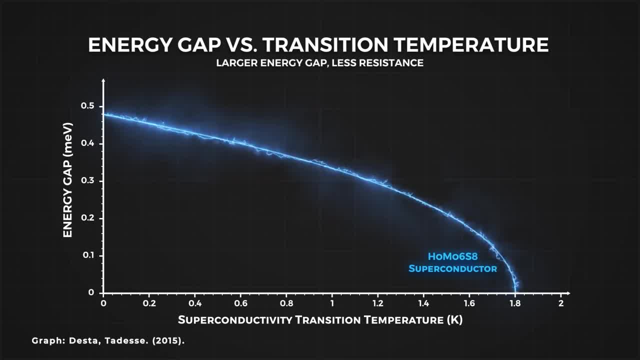 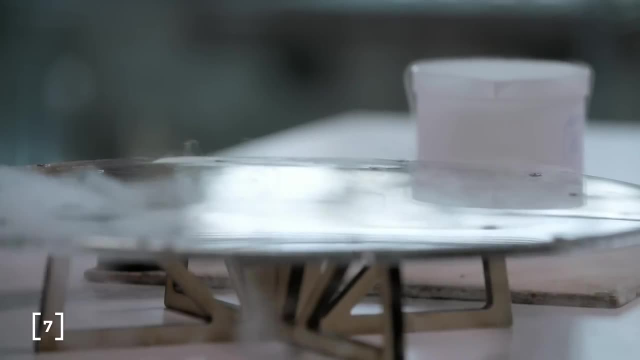 particle that, according to quantum mechanics, can only absorb energy at specific intervals. This cohesion creates an energy gap. Only particles with the right energy can interact with cooper pairs. This is why the crystals need to be cooled down to such low temperatures, Below 40 Kelvin- they don't have enough energy. 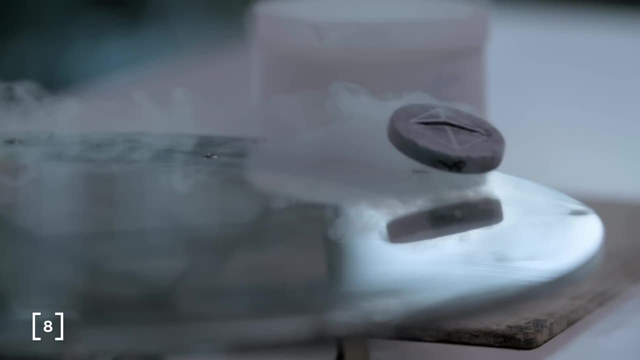 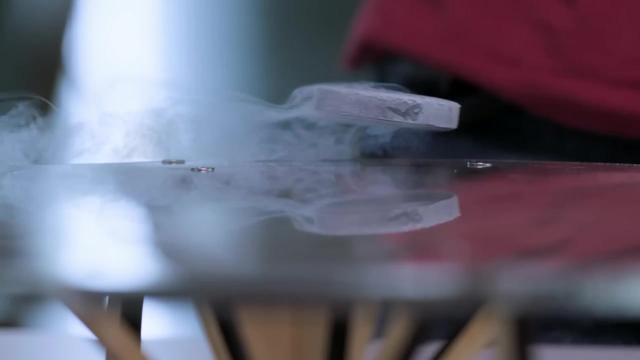 to interact with the cooper pairs, So electrons just glide along without interacting with the material, leading to no energy loss due to resistance. However, in 1986, a new discovery blasted this explanation out of the water, introducing the world to a new material that 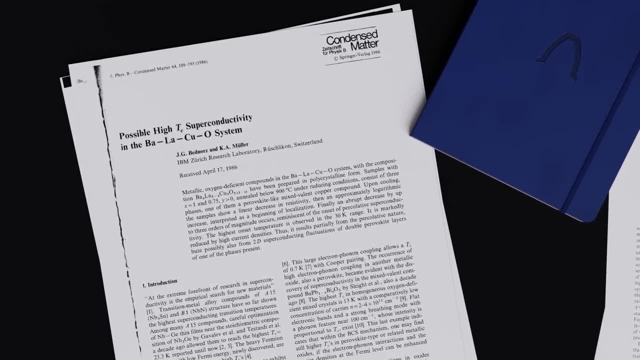 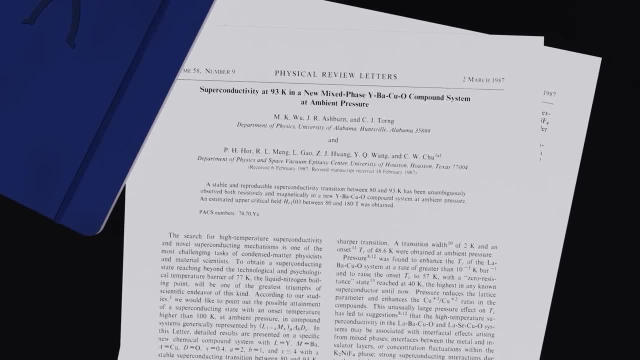 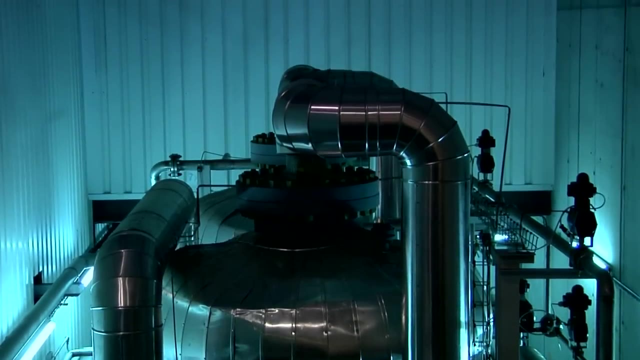 couldn't be explained. IBM researchers identified a class of ceramic materials that could display high temperature superconductivity. Based on their research, another material with a critical temperature of 93 Kelvin was found a year later. High temperature being relative, this is just over. 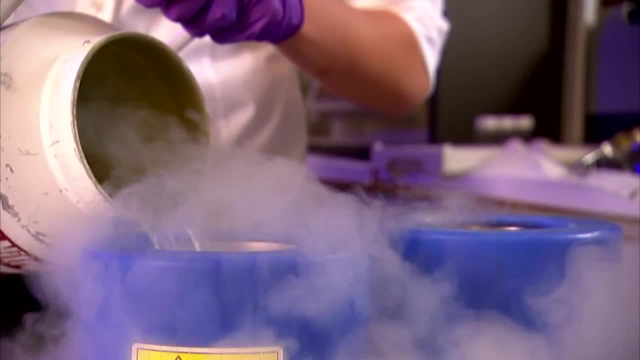 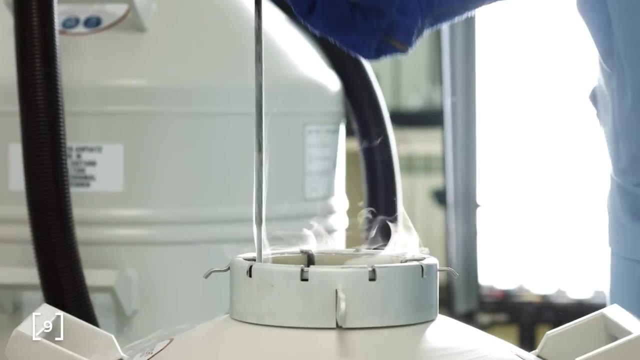 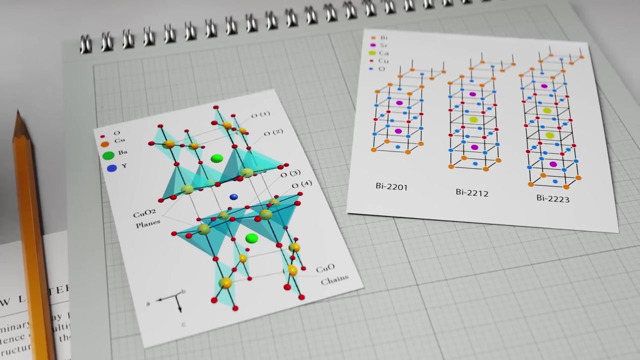 the boiling point of liquid nitrogen of 77 Kelvin- Still cold, but critically liquid nitrogen is affordable. To create 1 litre of liquid nitrogen it can cost as little as 15 cents. These materials have more intricate crystal structures involving layers of different elements like copper oxide. 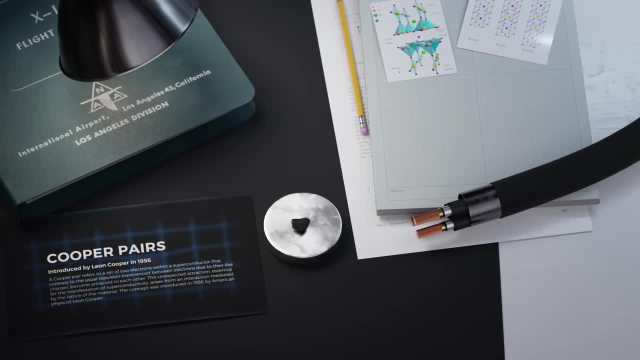 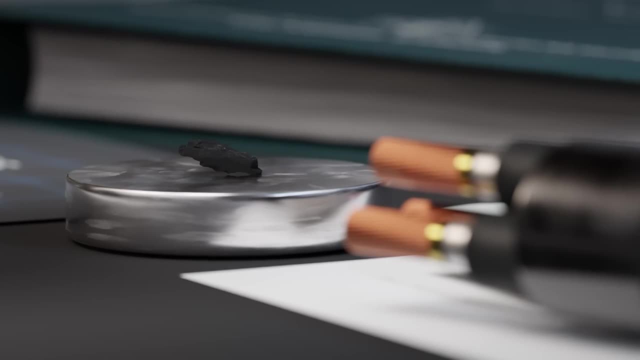 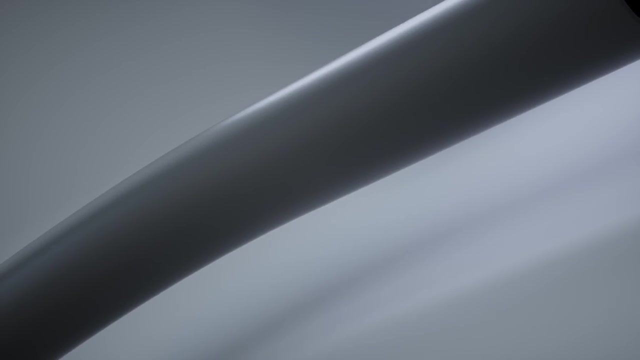 which contribute to their high critical temperatures. Because these materials couldn't be explained through conventional cooper pairs, they could not be explained through conventional cooper pair theory. A new category of materials was created, called unconventional superconductors, and we still do not fully understand how these materials work. But a lack of a full theory has 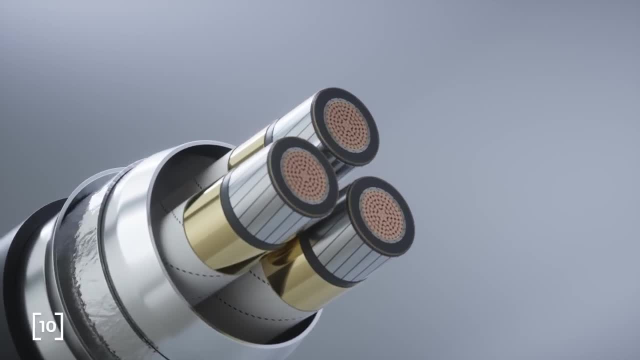 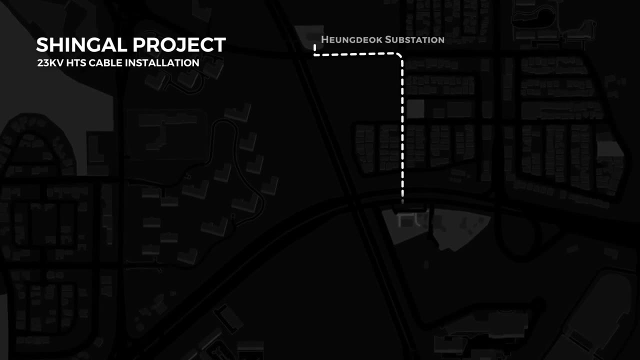 not stopped us from using them. We have created some unconventional superconducting transmission cables, like this one just south of Seoul in South Korea. It connects two substations that power a growing residential zone. They were already connected by two high voltage conventional. 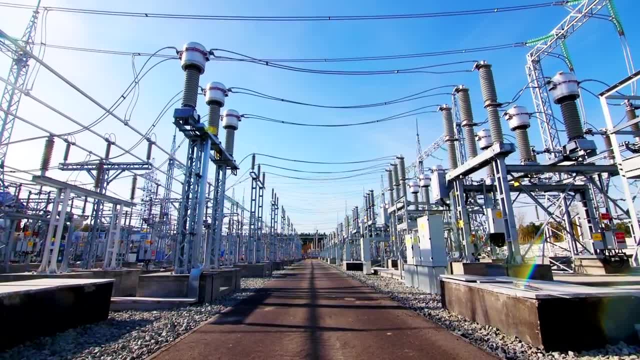 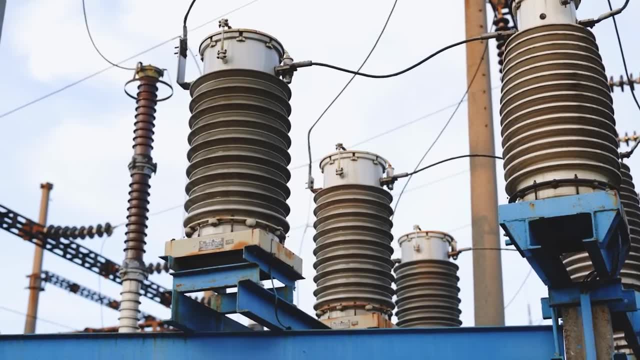 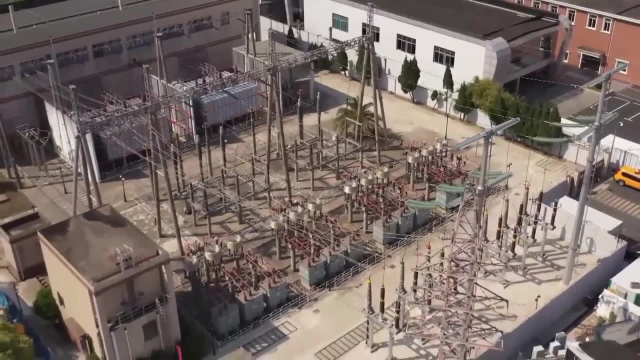 lines that were struggling to meet the increasing power demand, And adding another conventional cable would have required new transformers at each station to convert the high transmission voltage into the medium distribution voltage, and there was no space for another transformer. So the engineers turned to superconductors to solve the problem. We transfer power over longer distances. 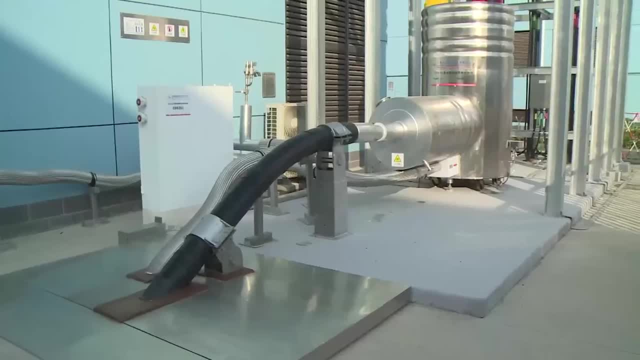 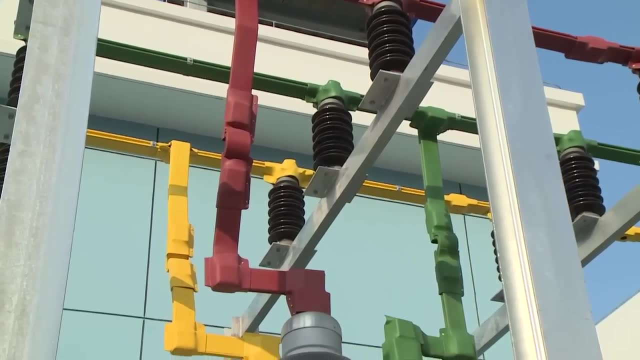 with high voltages to reduce power losses due to heat, But we can't use that voltage in our homes and step it down to a lower voltage using a transformer. However, if we didn't have to worry about losses, we could just transfer the power everywhere at the lower voltage. 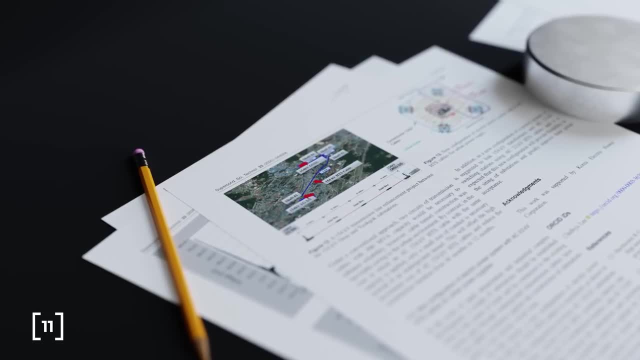 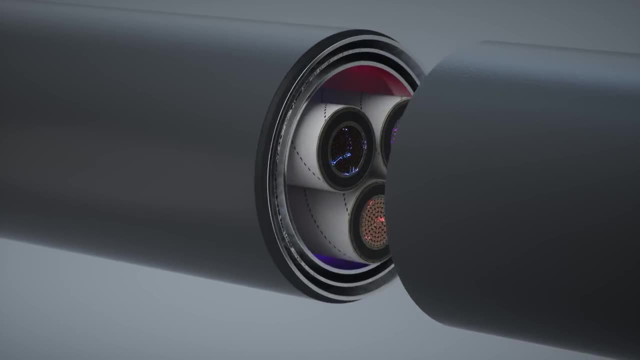 This is exactly what the superconducting line allowed and in 2019 it became the first commercial high temperature superconducting cable in the world. It's a 1 km AC cable which transports energy in three different phases. They used this configuration where. 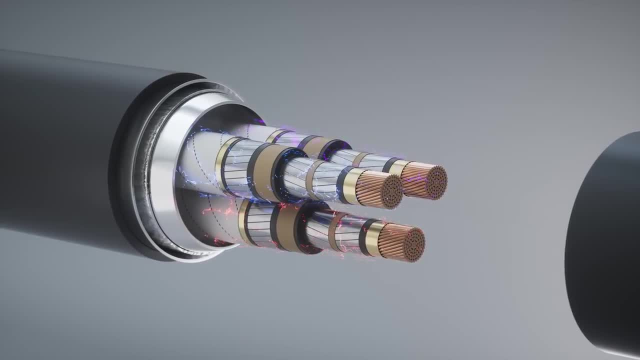 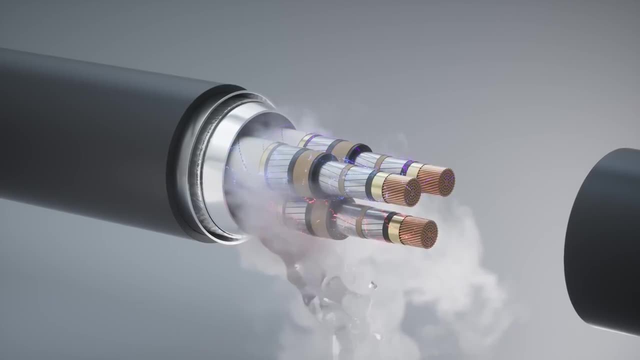 three cables are run parallel to each other to make it easier for the liquid nitrogen travelling by them. to keep them cool, Approximately half a kilogram travels by every second. The liquid nitrogen is pumped through at 66 kelvin To avoid losing heat. the cables are surrounded. 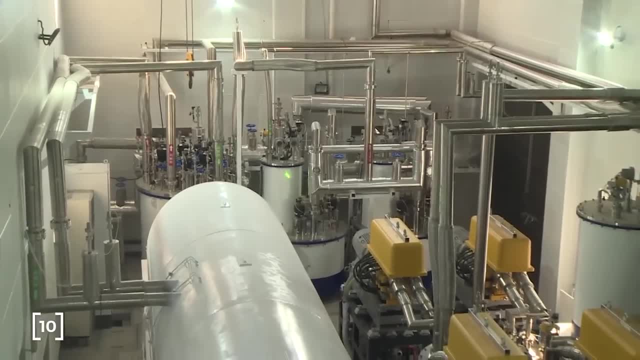 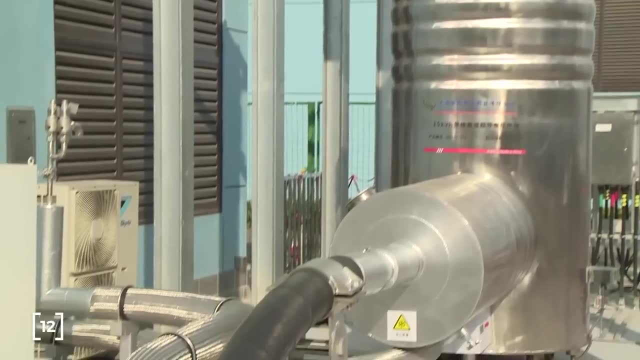 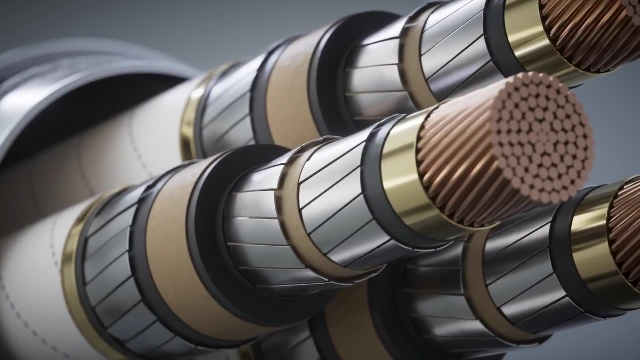 by a stainless steel vacuum chamber. Of course, some heat does leak in raising the outlet temperature by 3 kelvin, amounting to a 3 kilowatt energy loss, the same as 30 100 watt household fridges. One of the interesting problems facing this cable is the material properties of the 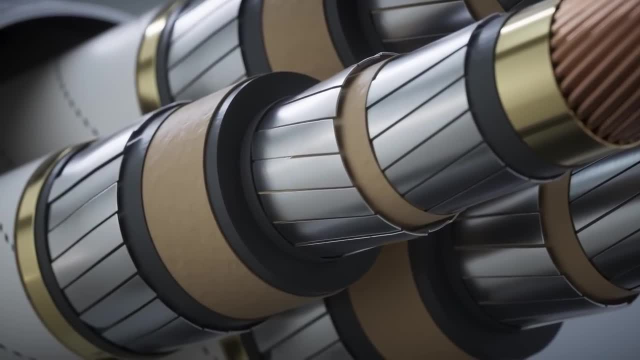 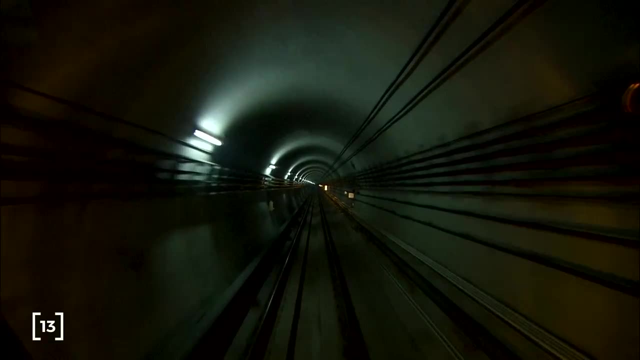 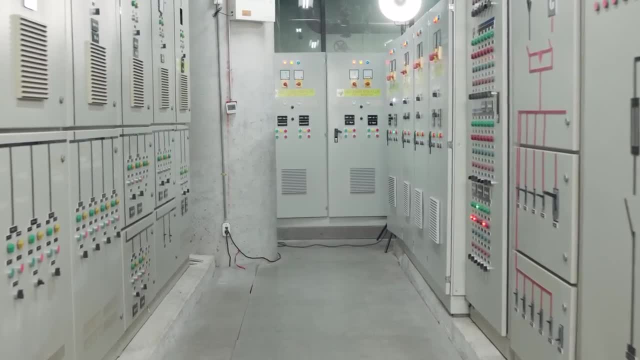 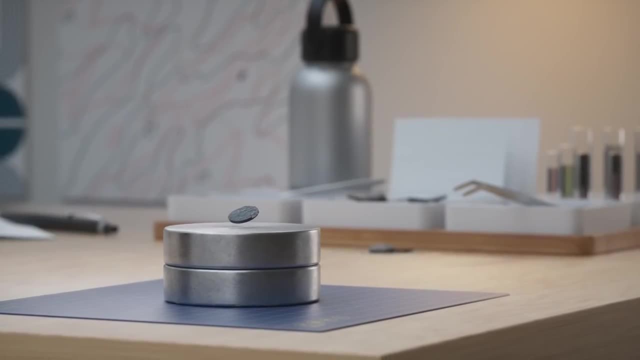 cost you a lot of money, while a traditional superconducting cable would cost you a lot of money. The South Korean project was a unique problem that needed a unique solution that justified the extra costs. This is why a room temperature superconductor would be game changing. 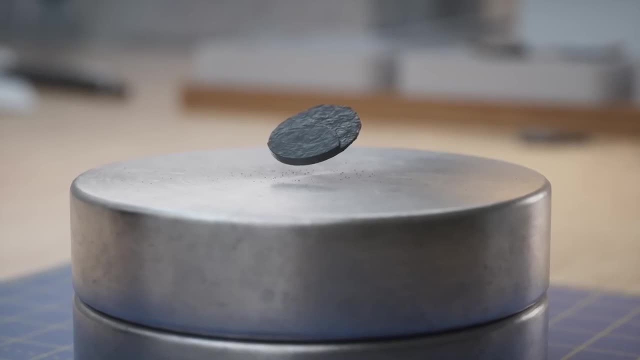 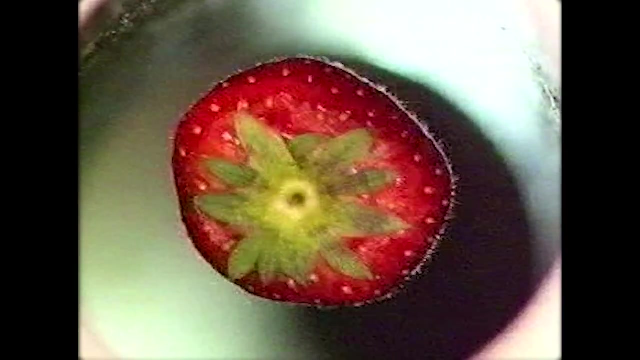 When the news of LK99 broke, images of the levitating material spread across the internet. But levitation doesn't necessarily mean superconducting. Other materials can levitate through a mechanism called diamagnetism. Water is a little diamagnetic, so we can actually levitate. 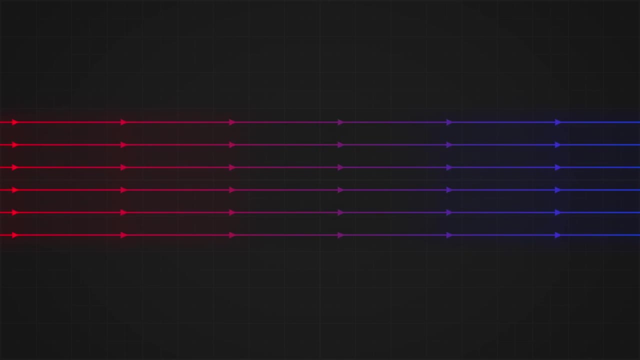 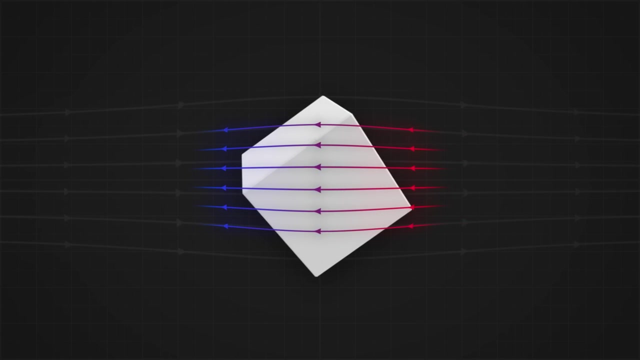 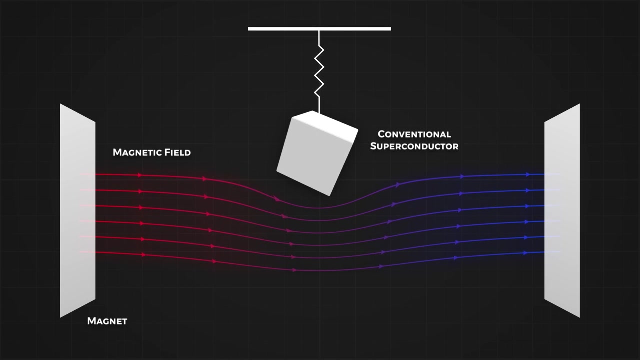 small animals with this effect. Diamagnetism simply means that when the material becomes magnetic, when placed in a magnetic field, its own magnetic field is in the opposite direction. Magnetic fields cannot be cancelled, so these materials just redirect the lines around themselves. This results in a measurable repulsive force between the material. 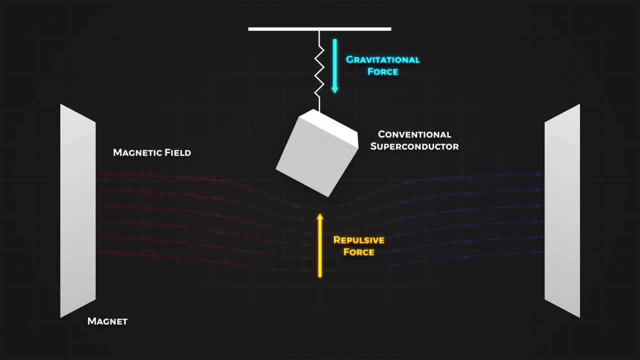 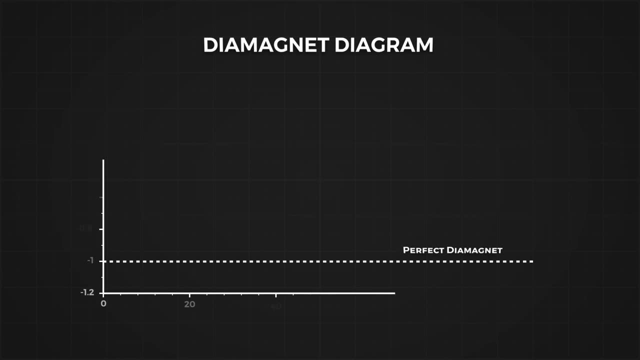 and the magnetic field. Quantifying this effect involves suspending the material with a force caliper in a magnetic field and measuring the change in weight caused by the repulsion. This is what the graph would look like when quantifying the diamagnetism of a superconductor: A straight line at high temperatures. 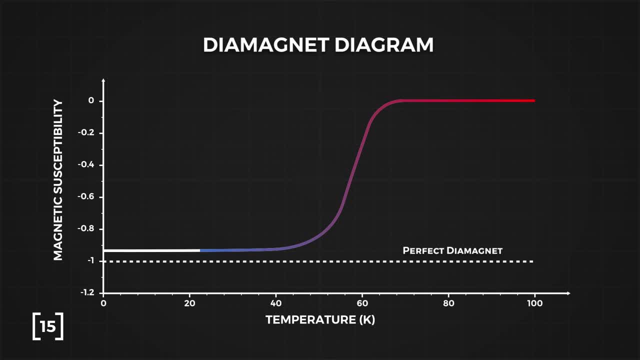 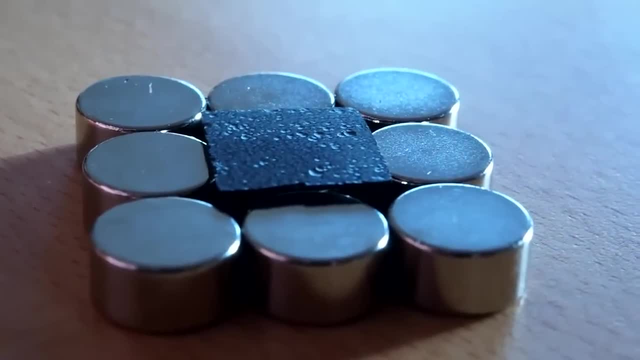 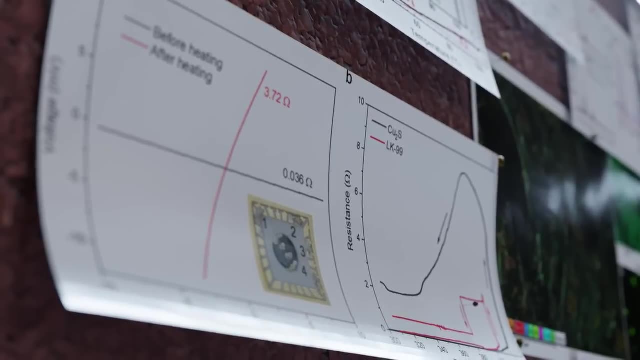 but a sharp change at their critical temperature, becoming a perfect diamagnet. At this point all magnetic field lines are expelled outside the material and the material just levitates above the magnet. This is called the Meissner effect. But even though we have tests like this, it doesn't stop researchers from lying. 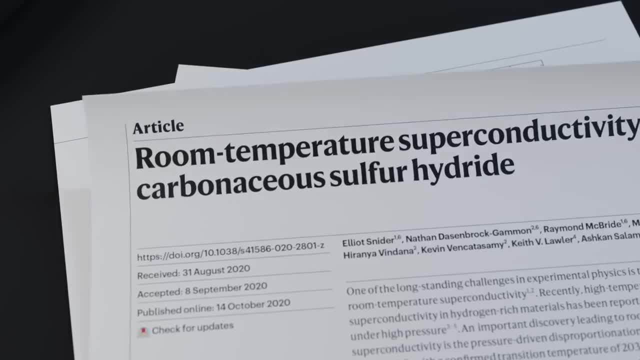 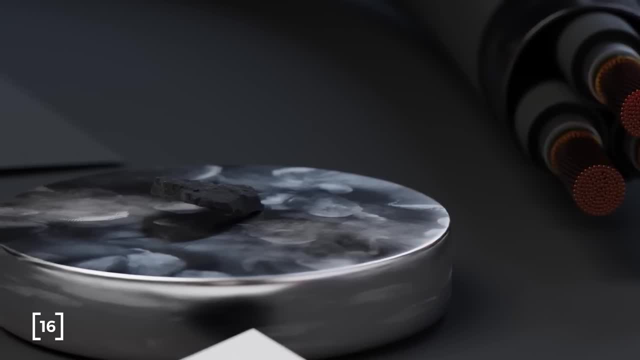 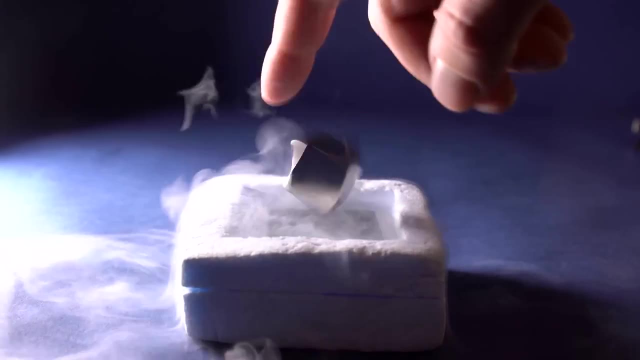 In 2019, a research team reported discovering a room temperature superconductor and backed it up with data showing perfect diamagnetism, But upon further examination, the data was found to have been copied from another paper. With so much world changing potential, researchers often rush to push their papers out as quickly as 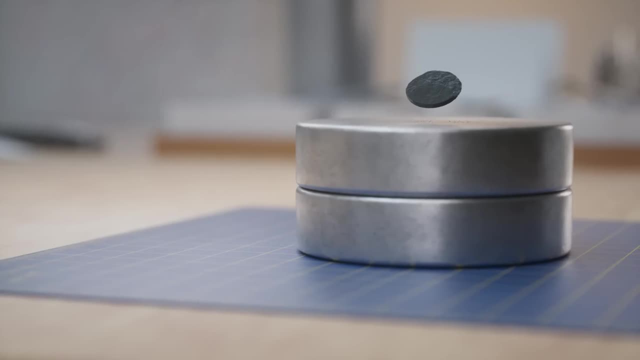 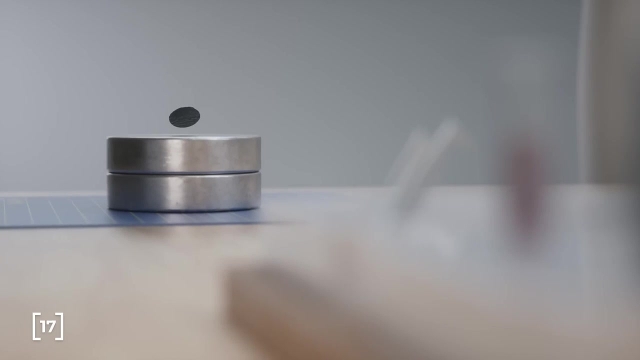 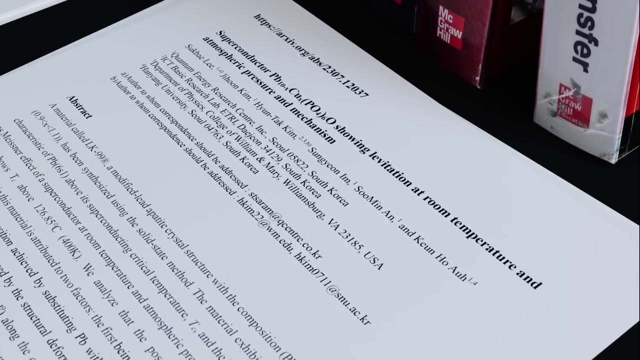 possible. This is why the scepticism was so high for the LK99 announcement. The South Korean team published their results on a pre-published website and it raised some red flags. The first paper posted on Archive had three authors. Two hours later, a similar paper was posted, but this time it had five- An odd choice. 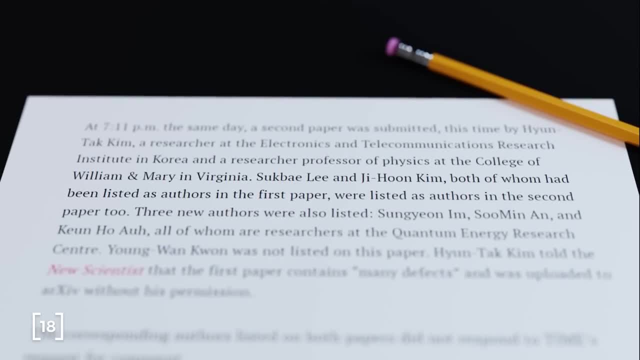 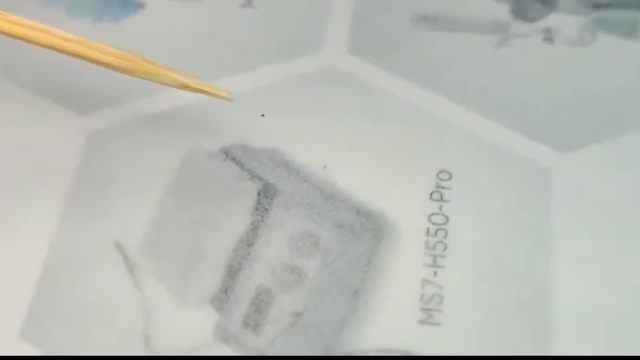 that seems to point to a fight for the recognition of the discovery. Later, one of the authors said the paper was full of errors and was posted without his consent. Fortunately, the team provided clear replication instructions and 11 labs worldwide have published preliminary results. 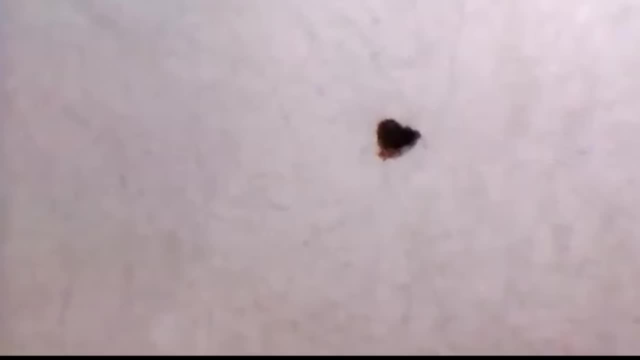 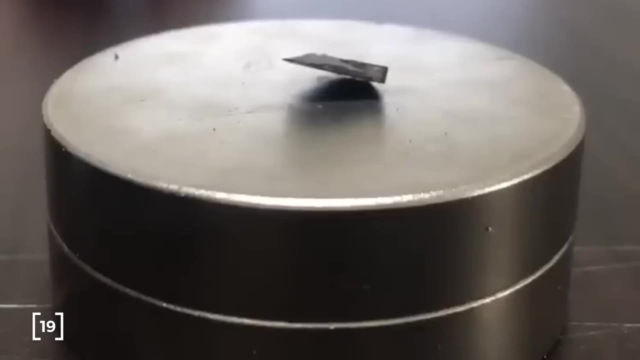 The first and most obvious piece of evidence are the videos of the material levitating on top of a magnet. LK99 definitely has some diamagnetism to it, but it's hard to say for sure. LK99 has some diamagnetic properties that have been replicated by other teams. This is the resistivity data, the 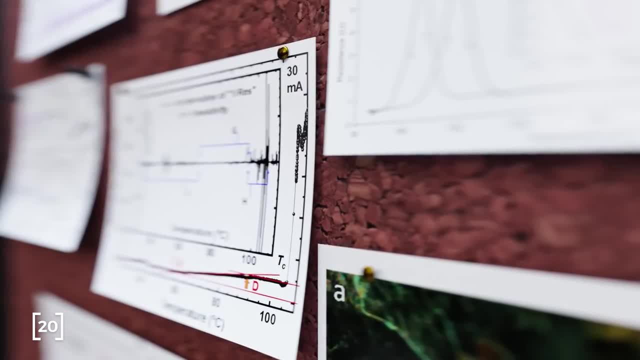 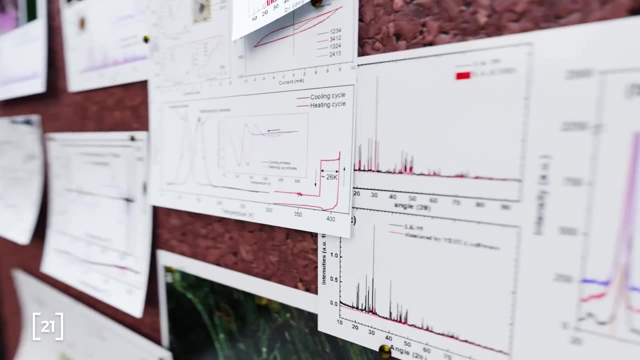 South Korean team presented A sharp drop in resistance around 380 kelvin. The temperature at which this happens in the replication samples varies from 100 kelvin to 400 kelvin and in all the samples resistance never truly drops to zero. The range of results points to. 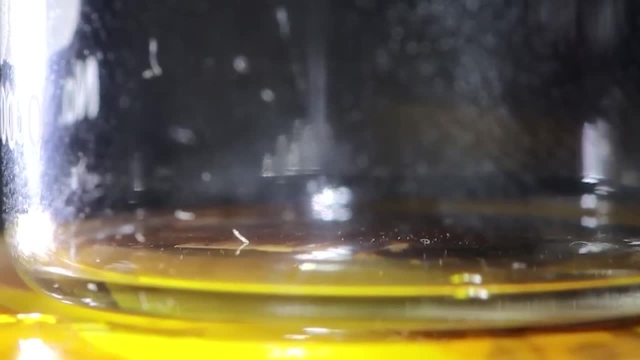 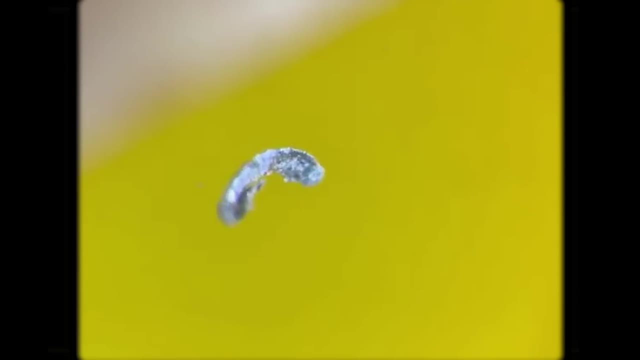 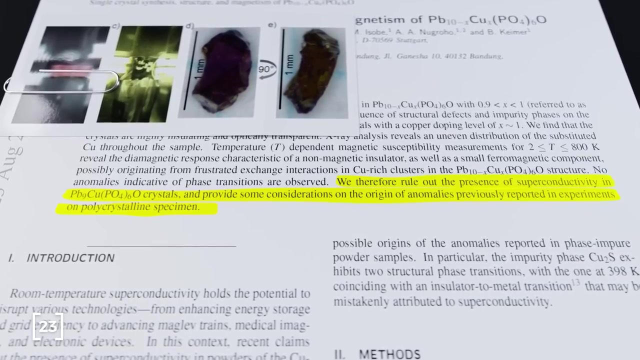 an impure material. So a German team created a sample of LK99 using a different process, One that gasses in a tube to remove the sample's exposure to impurities, creating a pure LK99 sample. It was transparent rather than grey and actually turned out to be an insulator with some diamagnetic. 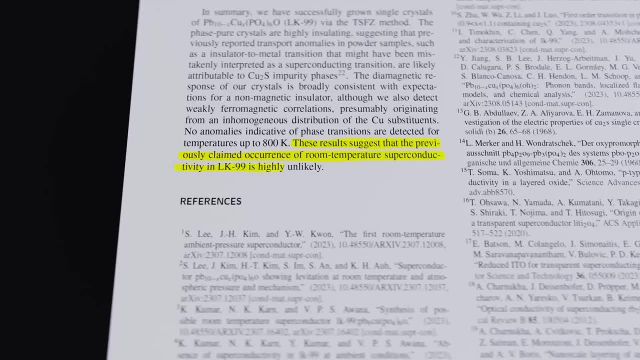 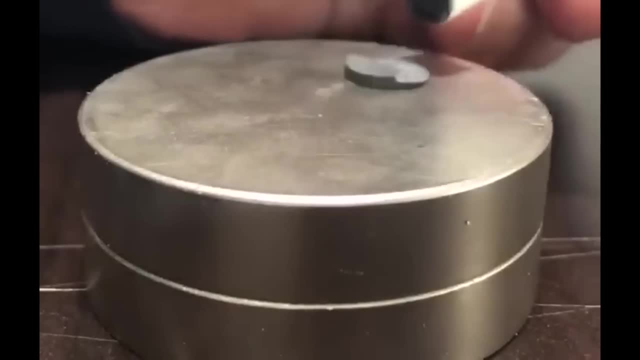 properties. All this evidence points to LK99 having some interesting properties, but it is not a superconductor. The world understandably got a little excited about the potential of this discovery. Being able to harness the power of superconductivity is a literal superpower. 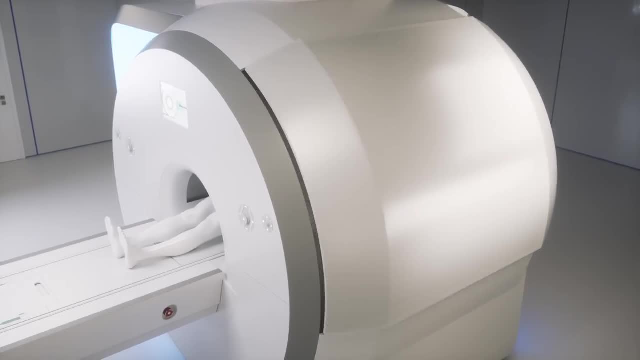 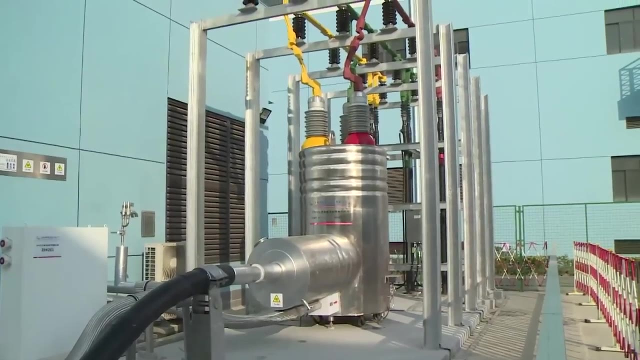 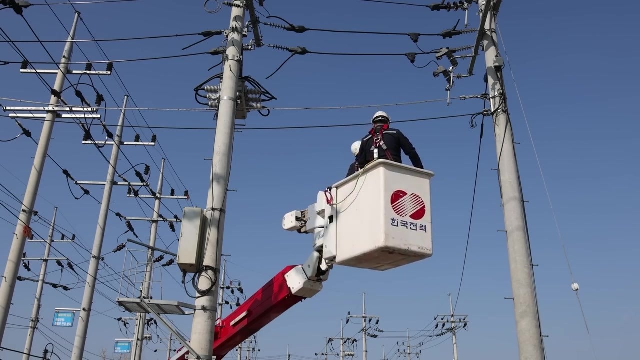 And we are still learning how exactly it works. It's astounding that we already have functional technologies like these high temperature superconductors in South Korea that make the technology vastly more accessible. For now, high temperature superconducting cables have some good use cases in dense urban centres like Seoul, where limited space and ever increasing 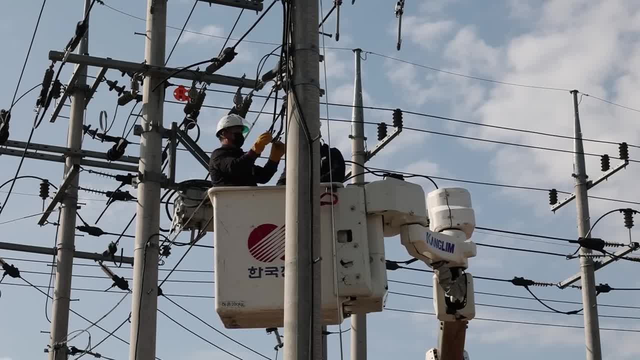 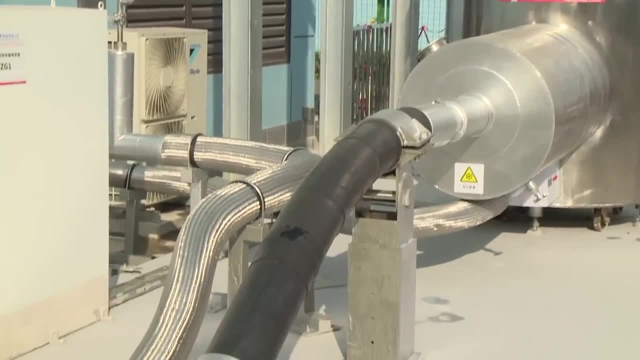 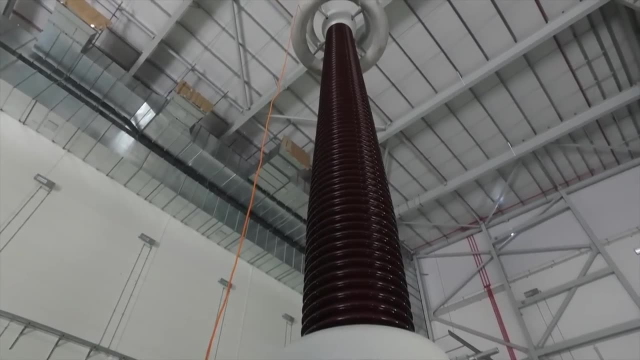 power demand opens the door to futuristic technologies And hopefully, with its success, prices can begin to lower as we figure out ways to lower the material and manufacturing costs while increasing efficiency. The world changing effects of being able to transport a large amount of electricity with no losses across further and further distances. 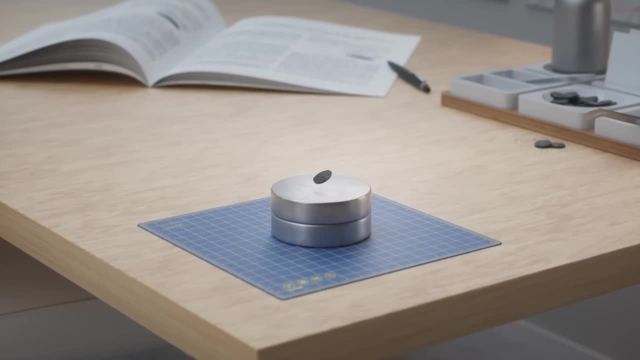 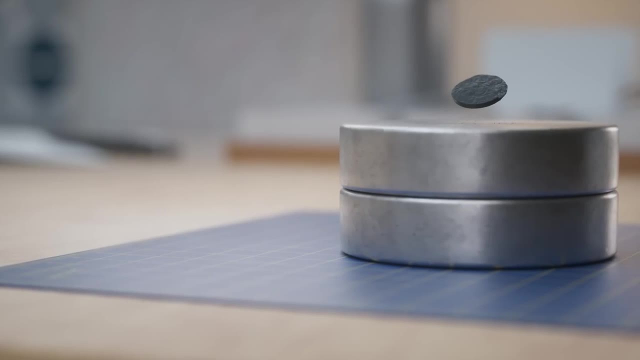 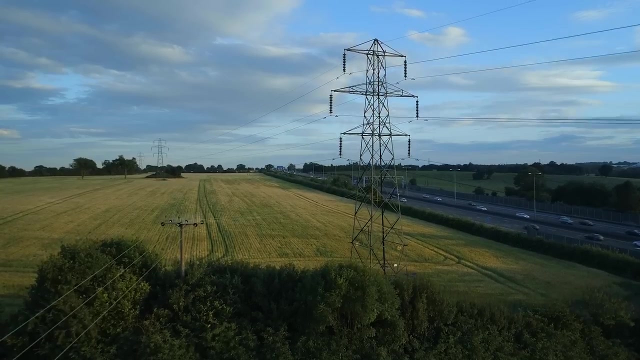 cannot be overstated. The enthusiasm of scientists who believe they made a world changing discovery is perfectly understandable. It would be a discovery that would mark their names in history forever. The electrical grid is incredibly complex. It's one of those subjects I'm oddly obsessed about Where others get excited. 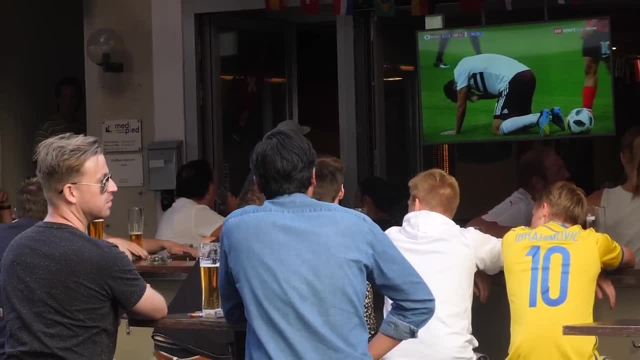 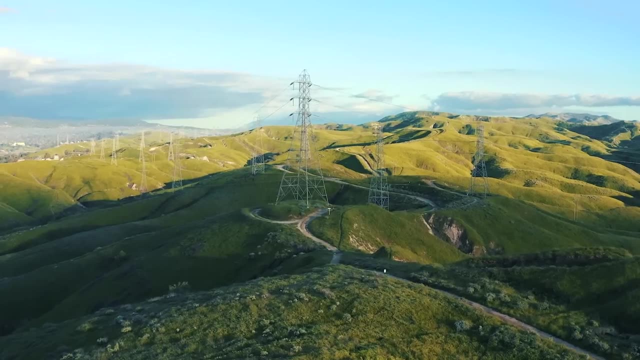 the conversation turns to the latest football game. I suddenly get more animated and join the conversation when the latest grid outage is discussed. Power grids are the world's largest machines, spanning entire continents, and are one of the major contributing factors to our country's economies. 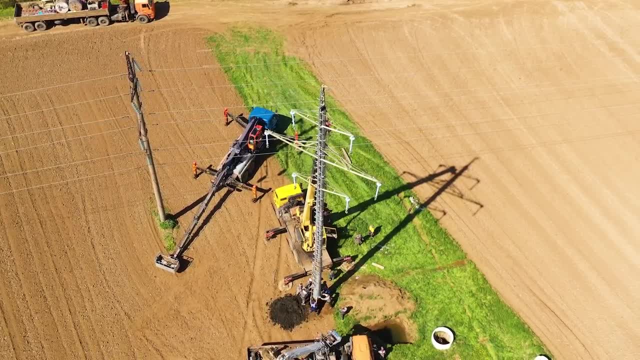 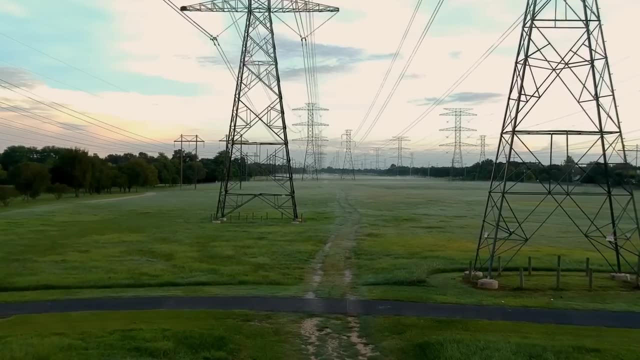 There are thousands of new jobs popping up every year in this industry. I have two friends who work in energy commodity trading, where they develop mathematical algorithms to buy and sell electricity for battery banks, Factoring in solar and wind fluctuations. power grids are the largest machines in the world. Power grids are the largest machines. 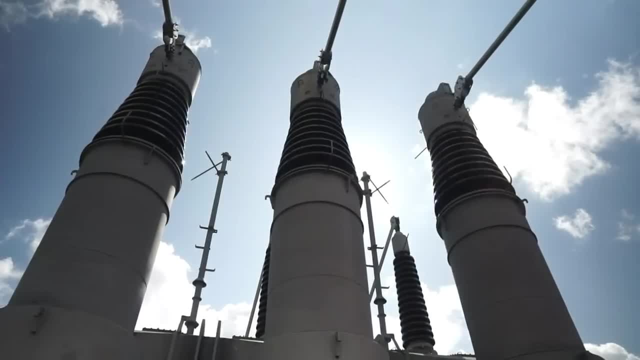 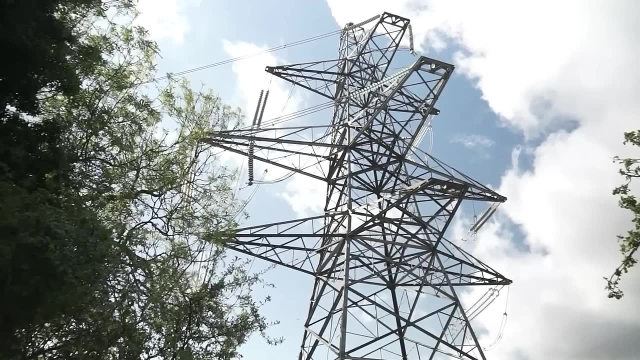 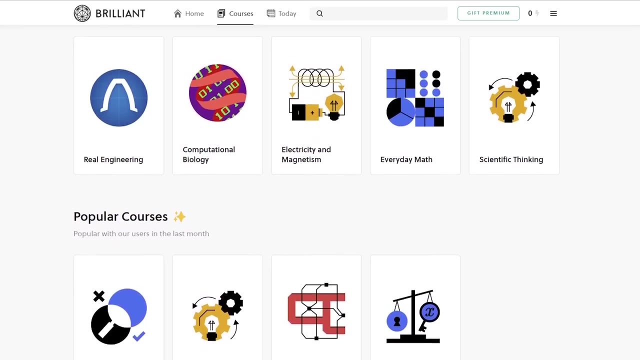 in the world. It's a fascinating and constantly evolving field. If that sounds like a field you could be interested in, there is actually a free and easy way to start learning about many of the core principles behind it. Brilliant: you have plenty of courses to get you started with a 30 day free trial.